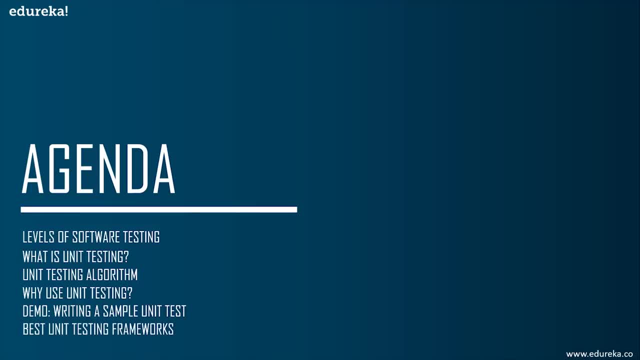 levels of software testing, and then we will move on to our today's topic, which is unit testing. there We will learn what unit testing is, why unit testing is really important. after that, We will do a small demo on how to write simple and easy to understand unit tests. 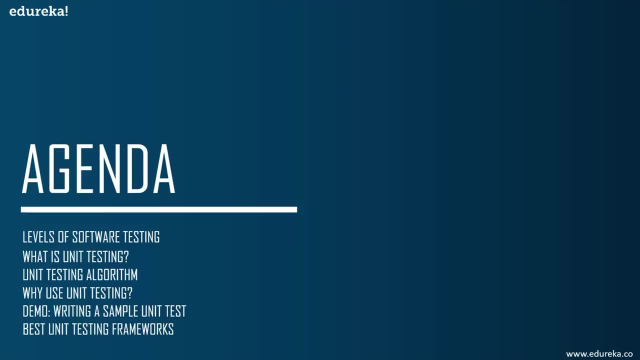 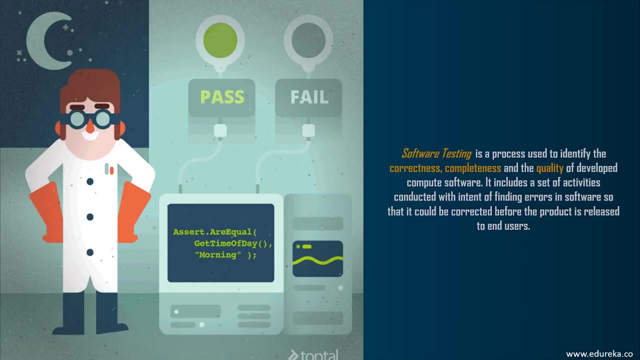 And finally, we will end this session by talking about best unit testing frameworks available in market. So I hope agenda was clear to you guys. Let's get started then. before software is released to market, It undergoes rigorous testing. I'm sure you guys know that testing is an integral part. 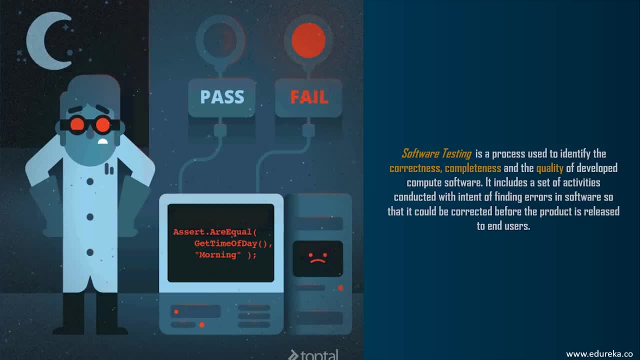 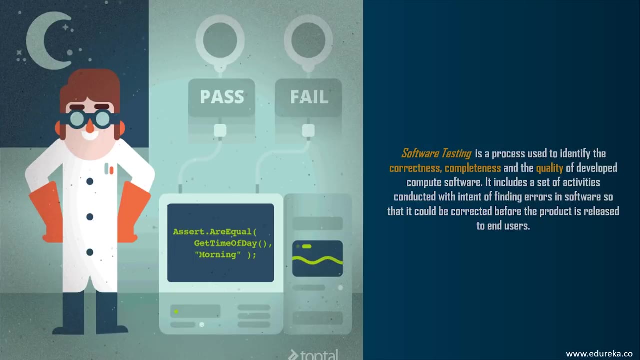 of any successful software project. software testing basically is the process of executing the software or any sort of application to find out if there are any bugs or some sort of errors in it. So before software actually goes public, programmers spend hours trying to find out every bug, that is, they check for any mistakes and problems in the design and 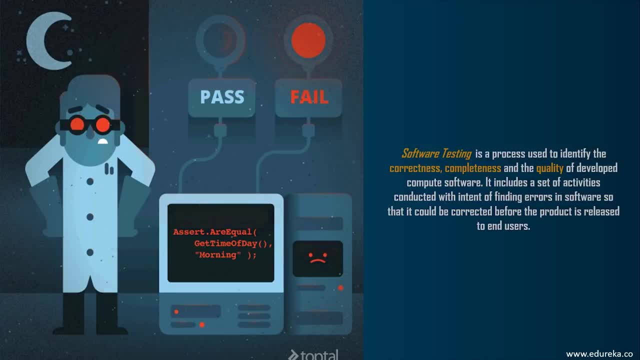 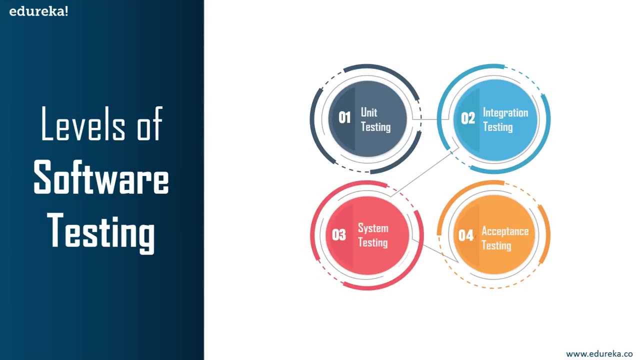 the functionality of the software. until then, product won't be available, Available for commercial use in the market. So, guys, there are four main stages of testing. So you need to perform this testing. only then you can say that your product is ready for the market. Those four levels are unit testing, integration testing, system testing and acceptance. 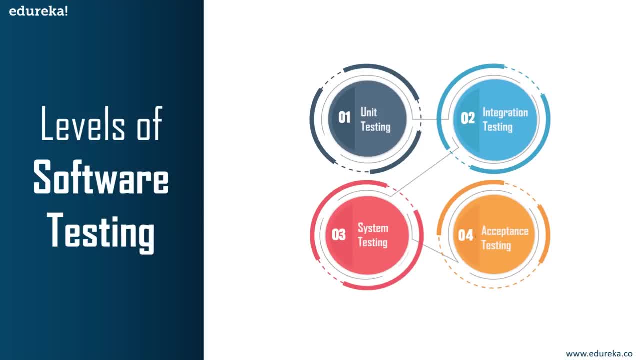 testing performed in the same order which I mentioned just now. So the first level of testing is unit testing. It's the micro level of testing. It involves testing individual modules or pieces of code to make sure that each part or unit is currently working. a unit can be specific piece of functionality, It can be. 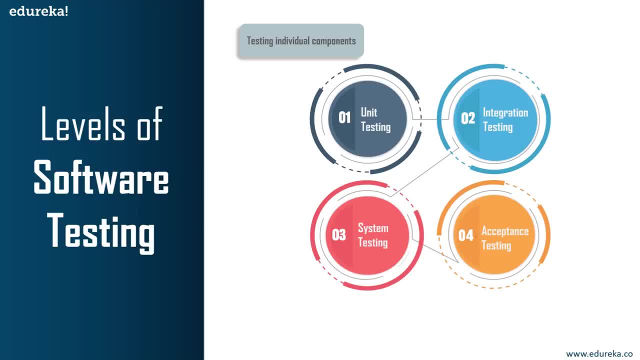 a program or a particular procedure within the application. It can be anything you want. unit testing helps verify internal design and internal logic and internal parts, as well as error handling. so that's unit testing, your first level of testing. after unit testing, We have integration testing. integration testing is usually done immediately after unit testing. 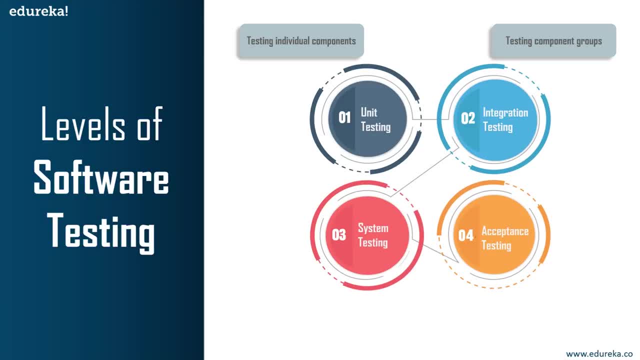 this level tests how the unit works together. Individual modules are combined and tested as a group. It's one thing if unit works well on their own, but how do they perform together? integration testing helps you determine that and also ensures your application runs efficiently without any error. 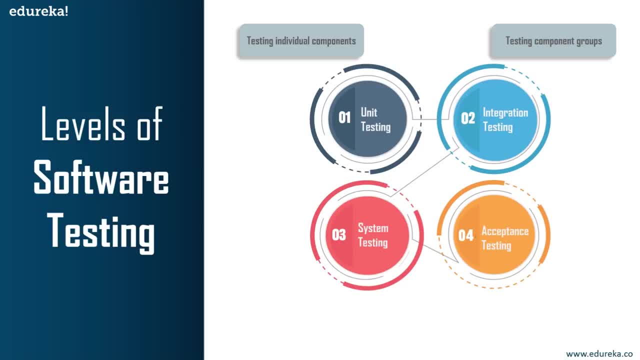 And lastly, it identifies interface issues between modules as well. So there are a few techniques that can be used for conducting integration testing. For example, you have something called Big Bang testing, top-down approach, bottom-up approach. Well, I'm not going to discuss all that here. 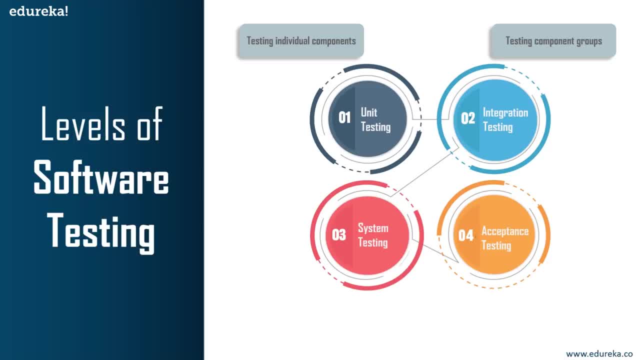 because they're out of scope of this session. Our main focus is on unit testing. after integration testing, The next level of testing is system testing. So, as the name actually implies, all the components of software are tested as a whole in order to ensure that overall product is working properly as you expected. system. 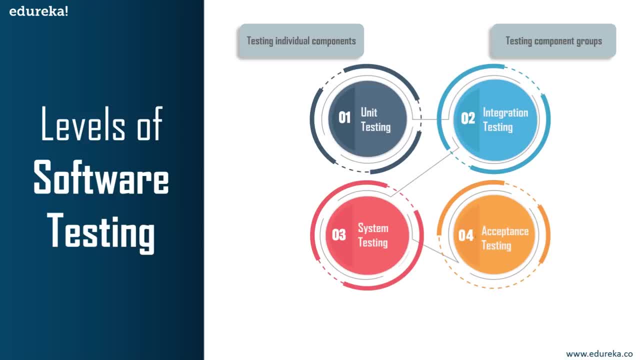 testing is particularly important because it verifies the technical, functional and business aspects of your software. There are dozens of types of system testing. for example, you have usability testing, regression testing, functional testing and many others. Well, if you want to know more about these type of testings, 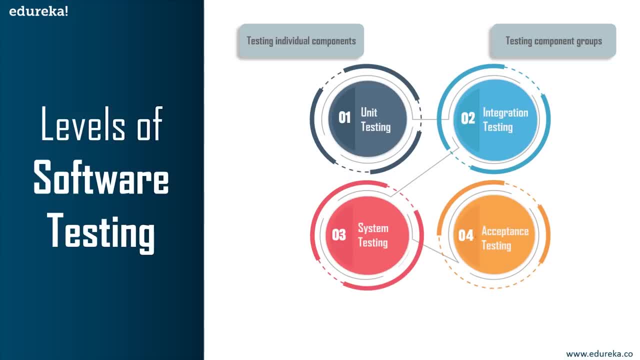 you can refer to the software testing playlist in a direct or YouTube channel. moving on this system, Testing is typically done by testing team and includes a combination of automated testing as well as manual testing, and final level of testing is acceptance testing, or u80. We call it that's user acceptance testing. it determines 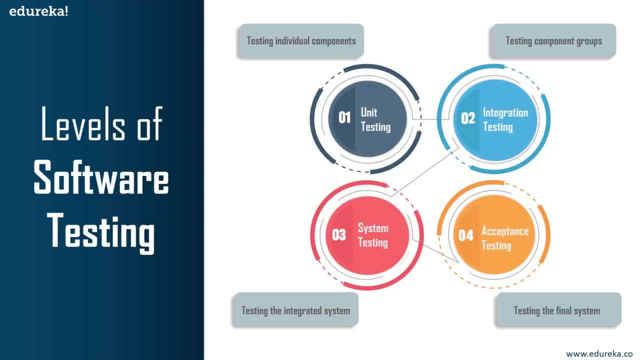 whether or not the software is ready to be released. Let's face it: requirements keep changing throughout the development process. right? You agree with me, right? It's important that user verifies the business needs are met before the software is being released into production. 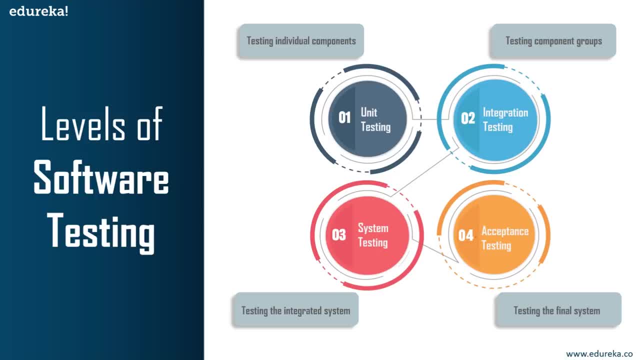 So, are the functional requirements met? are the performance requirements met? these are the questions that are answered during this level of testing. u80, or user acceptance testing, is the final say to whether the application is ready for the use in the real life or not. So, guys, these are four levels. 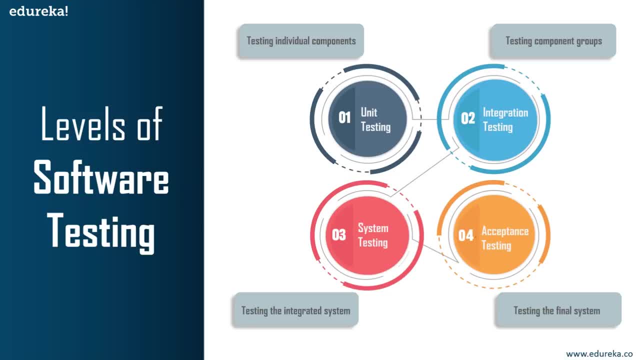 Of software testing. each level of software testing has a particular purpose and provides value to the software development cycle. Some levels are their own type of testing. For example, unit testing includes just that, unit testing. but integration testing can include many types of testing. So, guys, you can't mix up these levels. 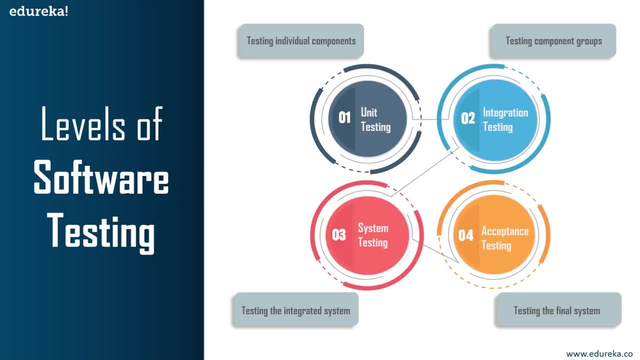 as you want, during development stages. There's a logical sequence that should that you should stick to in order to minimize the risk of bugs cropping up just before the launch date of your software. In today's session, We will be discussing particularly about unit testing. 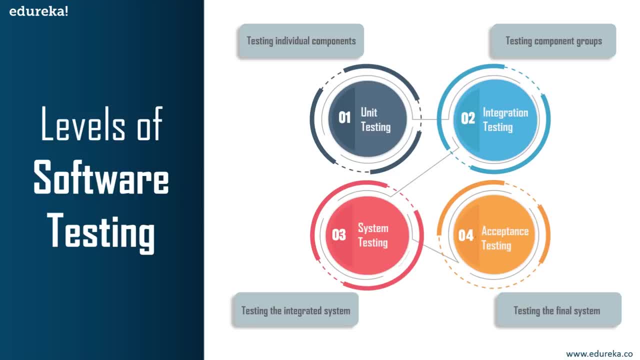 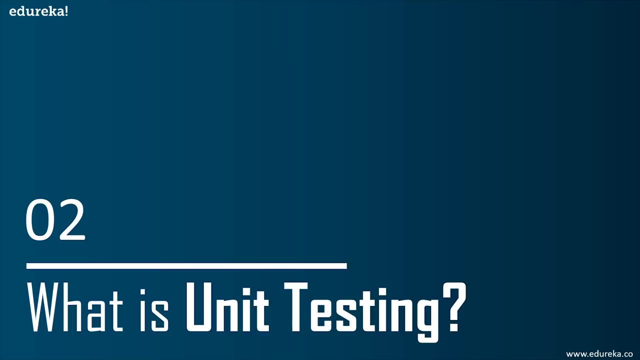 but before we get started setting up our environment and writing any code, let's Define exactly what unit testing is, Why is it's worth doing and how to get started and incorporating it in our software projects. So let's get started there. So the most basic type of testing is unit or component tested. 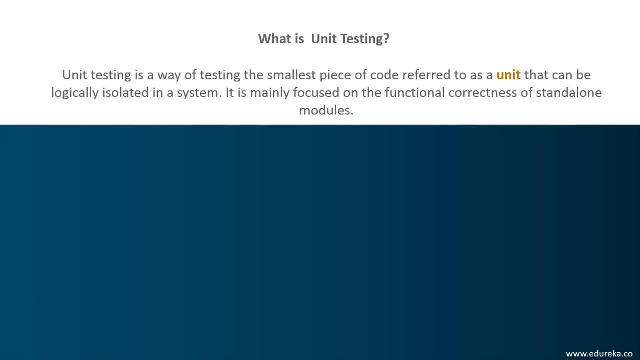 The goal of unit testing is basically to segregate each part of the program and test those part individually to check if they're working properly or not. So it isolates the smallest piece of testable software from the remainder of the code and determines if it behaves. exactly as you expected. 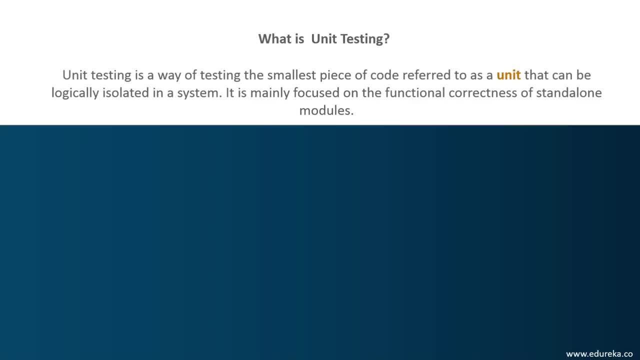 and according to your requirements or not. Generally, those small pieces of software that have been telling before are usually referred to as unit. So this unit can be almost anything you want it to be. It can be a line of code, It can be a method or a class or some sort of program. 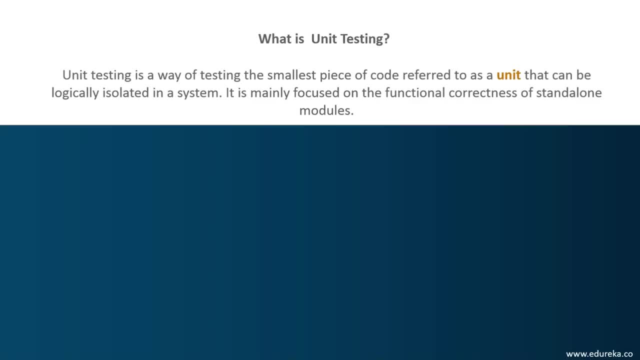 or a part of application Program, anything but smaller the unit is. it's always better smaller test give you much more granular view of how your code is performing at basic level. There is also the practical aspect that when you test very small units, you test can run very fast. 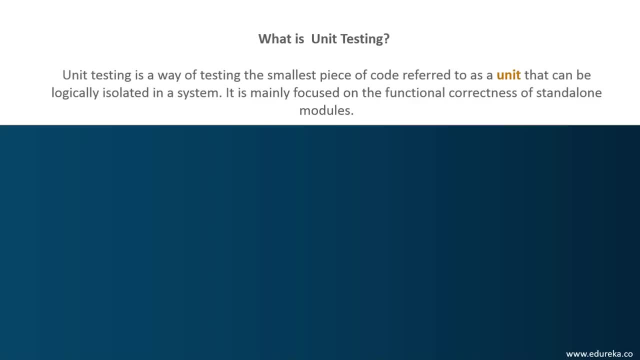 like a thousand test and second, fast that fast. Well, here's a simple example to help you understand what a unit can be or how unit testing is. so consider the simple code. Well, I have a simple function or method here. the function, as you can see. 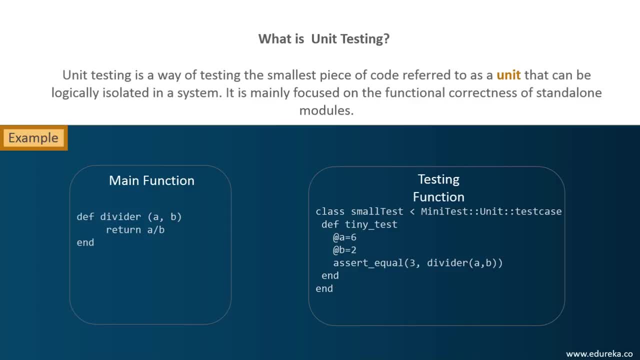 the main function. it's performing division operation. It's accepting two parameters, a and B, and it's returning the value that you get after dividing a by B. and next comes the testing function. as you can see, the testing function is written in Ruby. Well, the language doesn't matter the language. 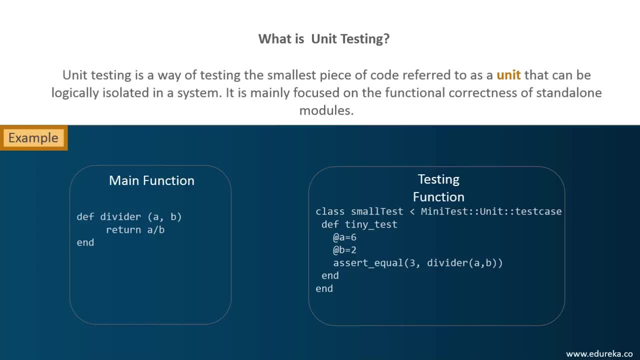 whichever you're comfortable with, you can use that. Anyway, as you can see, I have two variables, a and B, and I'm assigning values 6 and 2, and in the assert equal function, I'm calling the divider function and I also have the first parameter. 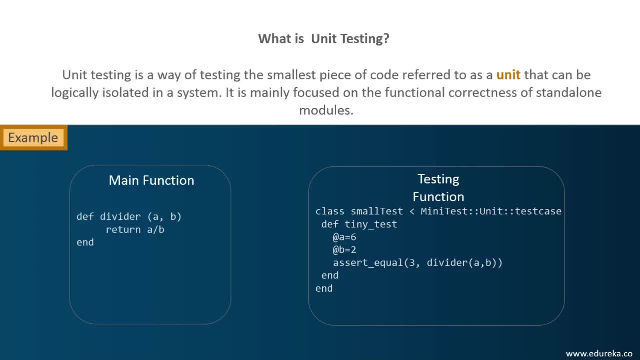 which is the value which I'm expecting that the division function should give it to me. So the value which I'm expecting is 3 and I'm passing the function and parameters to that function. So after dividing a by B, which is 6 by 2, I get the answer 3. 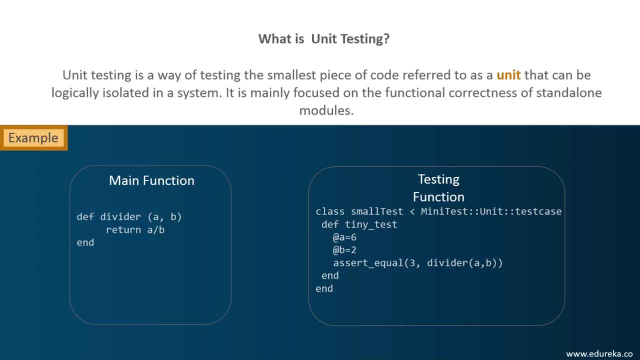 and assert equal functions tells me that 3 and 3, the expected answer and the actual answer I got, are the same, So my function is working properly. Well, this is a positive case. You can also do that with the negative case, as in. you can just change the 3 expected value to 4. 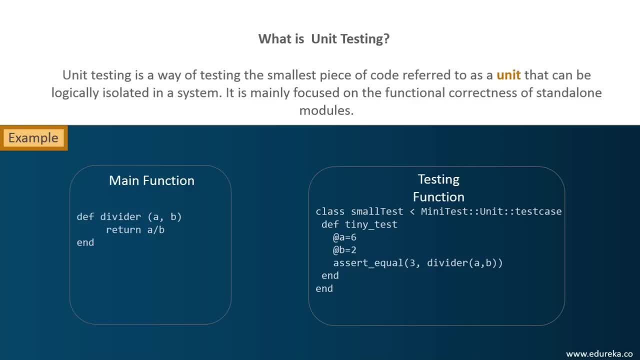 and see if the assert equal function returns to the actual answer. It says that your test fails. It means that the expected answer and the obtain answer not the same. So that's how you perform a testing on small unit which is a part of your entire program. 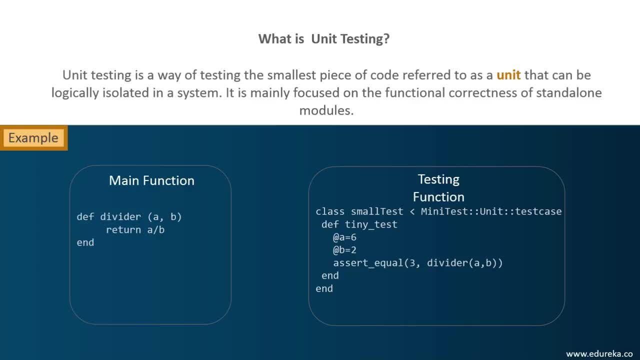 So you're, the small unit is division function. So, like I said, a unit can be almost anything you want to be. It can be a line of code, or it can be a method, or it can be a class. So this is very basic example. 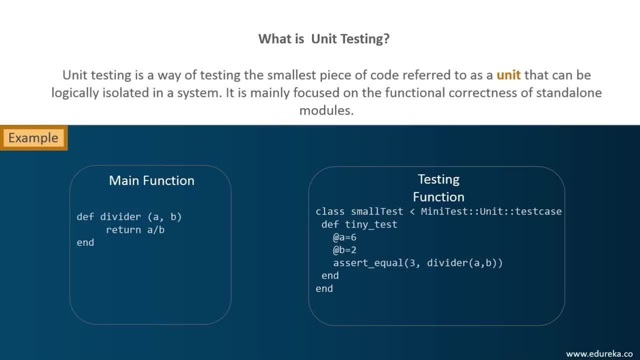 but I'm sure it gives you an idea of unit testing right? So, guys, unit testing is usually performed at the earliest stages of development process, like I said earlier, and many cases it is executed by the developers themselves before handing the software over to testing T. 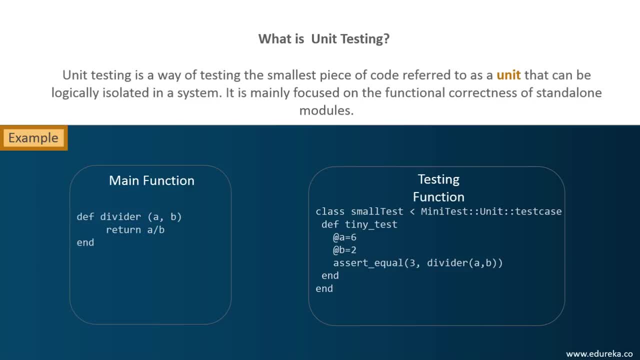 One of the biggest benefits of this testing is that it can run every time a piece of code is changed, So that way you can resolve if there are any errors very quickly. and since you're dividing your code into modules here, you can reuse your code. 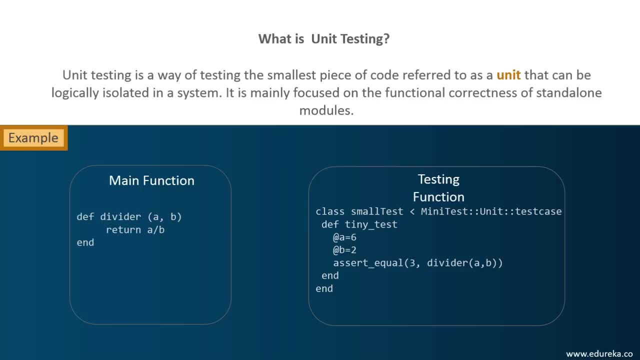 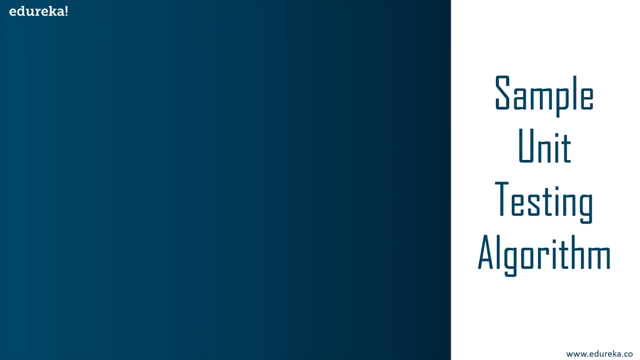 and testing becomes much easier and efficient and your product is well worst in the market. now, to understand unit testing better, Let's go ahead and see a simple algorithm. So you start writing your test, So you add your test to those test suit, then you run the unit test. if the test passes, 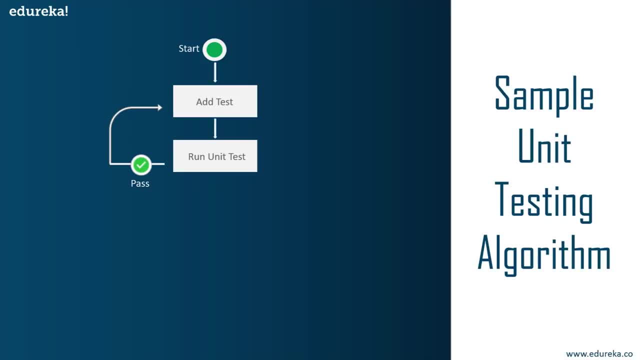 then you add one more test or add it to the next level of testing. in case your test fails. What you do? you make the necessary changes and you run unit test again, and after you run your test again, if it fails, then you make changes again. 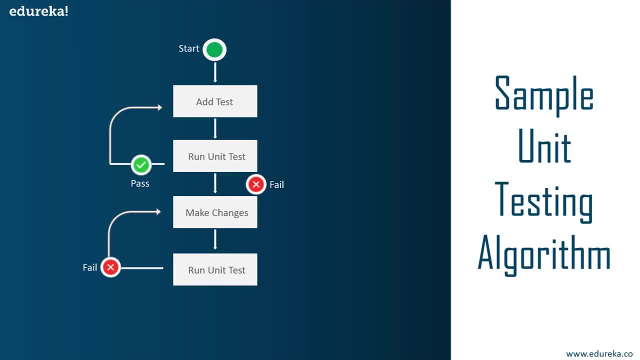 and you repeat the cycle until the code which have written is perfectly working and it's returning the value that you're expecting or the results that meets your requirement, and suppose, after making changes, if your test passes, then you can add it to the test suite and move it on to the next level of testing. 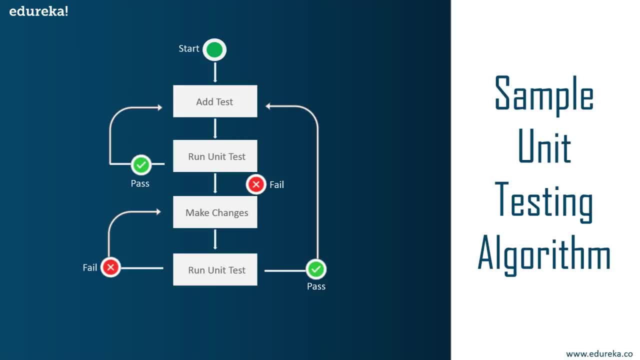 So once you are sure that all your tests are working properly- it means their test suit is perfect and your product is working properly- You can stop unit testing and perform next level of testing. very simple, right? this type of basic testing offers lot of advantages, guys. 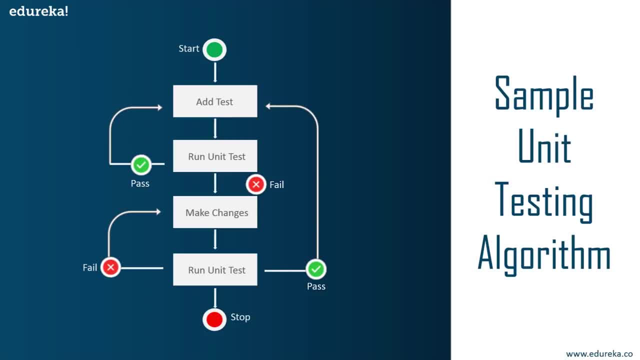 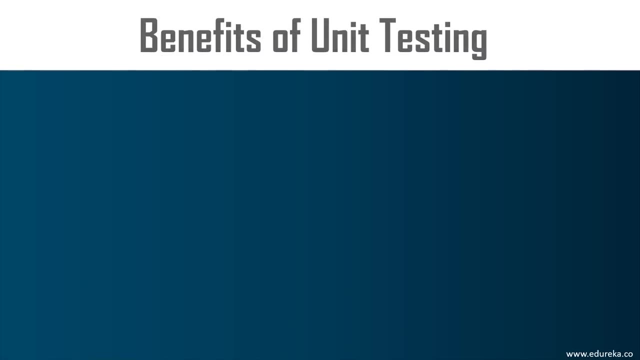 unit testing provides numerous benefits, including finding software bugs, facilitating change, simplifying integration, providing a source of documentation and many others. So let's take a look at them right now in more detail. So here are the benefits of using unit testing in software development cycle. 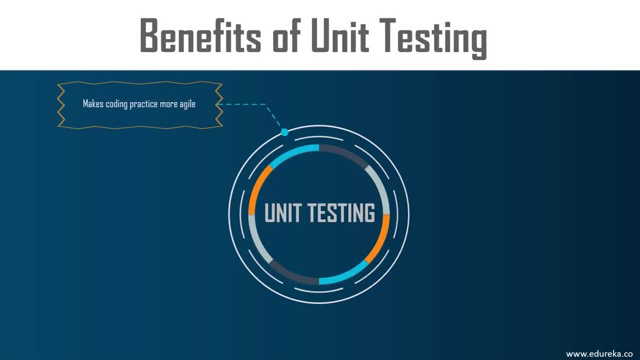 So, first of all, it makes coding process more agile. when you add more and more features to software, You sometimes need to change old design and code. I'm sure you agree with that. However, changing already tested code is both risky and extremely costly if we have unit test in place. 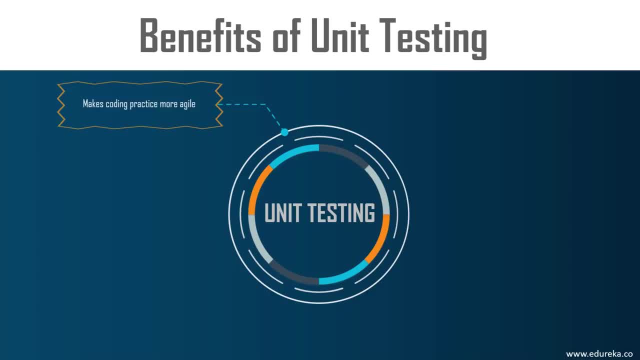 then we can proceed for refracting very confidently, because we know that each part of a code is working properly. So code completeness is very important in software testing, especially agile process. So running unit test can demonstrate code completeness. So unit testing makes code practice more agile. 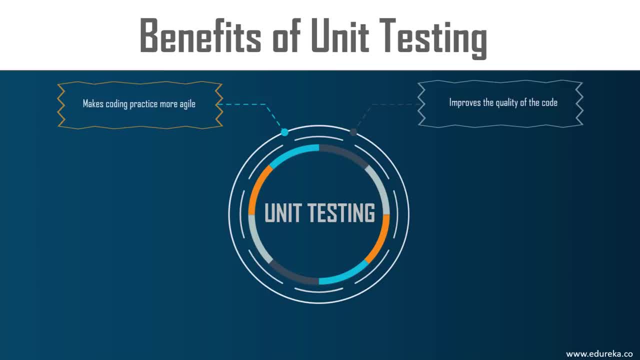 and very simple. Secondly, unit testing improves the quality of your code. It identifies every defect that may have come up before the code is sent further for further testing. So writing test before actually coding makes you think harder about the problem. It exposes the edge cases and makes you write better code. 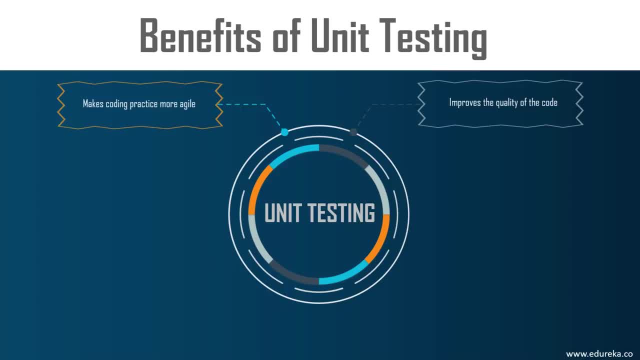 Also, the code that you've written is since divided into modules. that becomes reusable. This means that codes are easier to reuse when you perform unit testing. unit testing also helps find software bugs early, since unit testing is usually carried out by developers, Who test individual code before integration issues can be found. 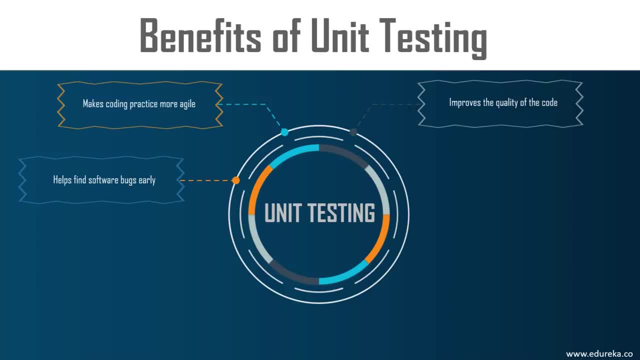 very early and can be resolved easily without impacting other pieces of code. So that one day of detecting any errors in software early in the day is that. by doing so, the team minimizes software risk and avoid spending too much money in time. unit testing also facilitates changes and it simplifies integration. it allows 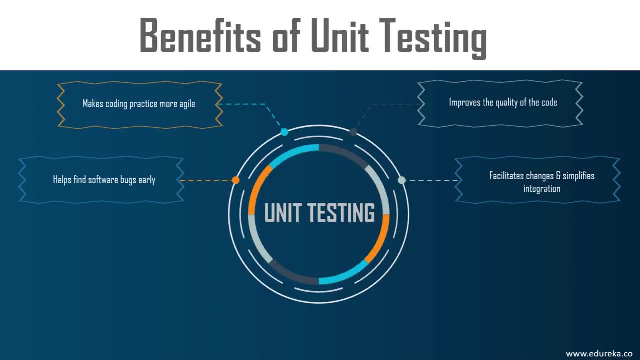 programmers to refactor code and upgrade system libraries at later date and make sure that the module still is working properly. Unit testing helps with maintaining and changing the code. it reduces the defects in your newly development or the newly developed module of your code. It reduces parks when changing the existing functionality, as 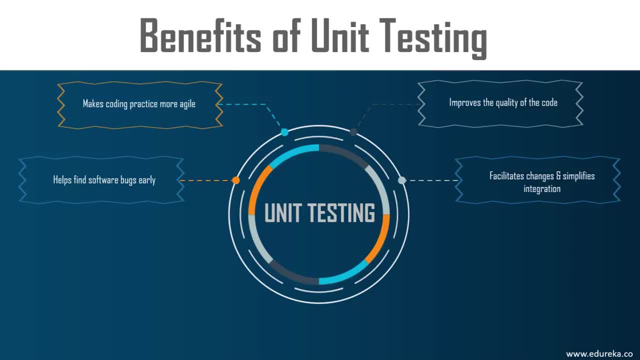 well, unit testing actually verifies the accuracy of each unit after what the units are integrated into an application by testing parts of the application via unit testing. So basically it makes integration much more better. It provides documentation to developers. So code documentation is basically a drag and it shows mostly how little code documentation 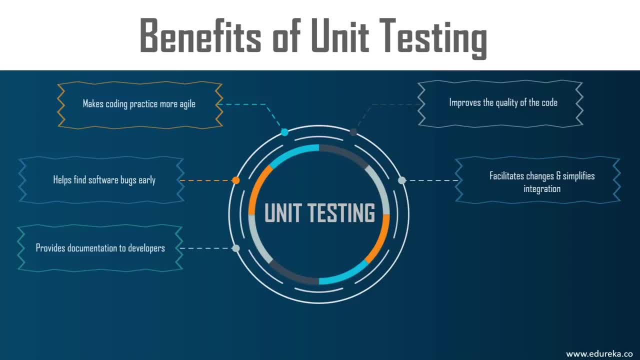 gets written. unit testing can make the documentation burden a little easier by encouraging better coding practices and also leaving behind the piece of code that describe what your program is actually going to achieve. unit testing also makes debugging easier and quicker. It helps simplify the debugging process. 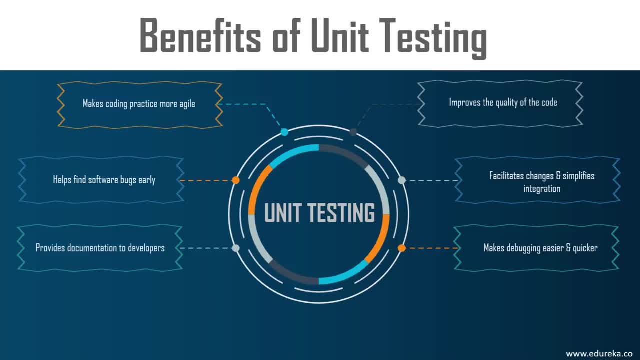 If a test fails, then only the latest changes made in the code need to be debugged. It's easy, right? It helps create better software designs. writing the test first forces you to think through your design and what it must accomplish before you actually write the code. 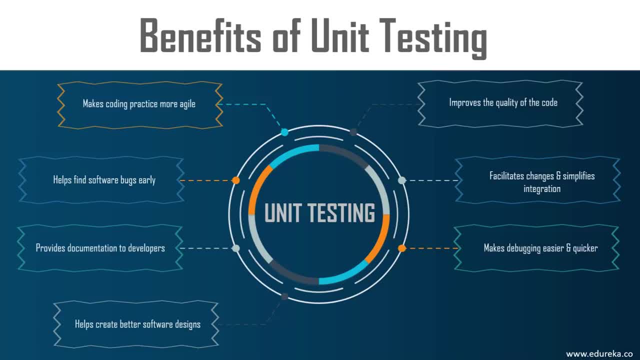 This not only keeps you focused, It also makes you create better designs. So that way, you're sure that the code you write will perform the right thing at the right time. And, lastly, it reduces testing costs, since the bugs are found early. unit testing helps reduce the cost of buck fixes. 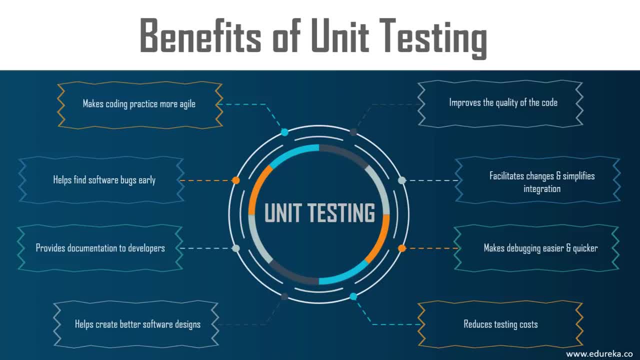 So just imagine the cost of buck found during the latest stages of development. You will have to modify the entire code of your project. that sounds really tiring and waste of money. So performing unit test saves you a lot of money and effort on your part. 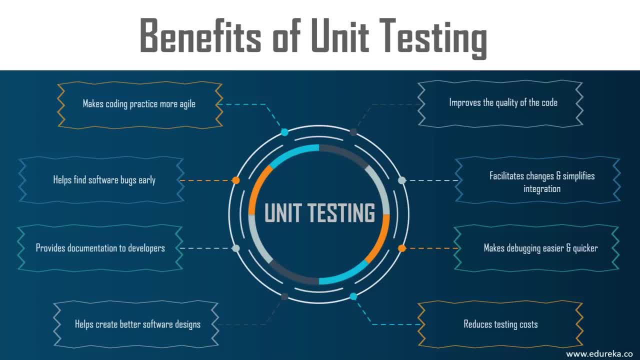 So, guys, these are a few benefits of regression testing. I'm sure there are others as well. Make sure you research on it and learn more about them. So there we go, guys. I hope you're convinced as to why you should use unit testing. 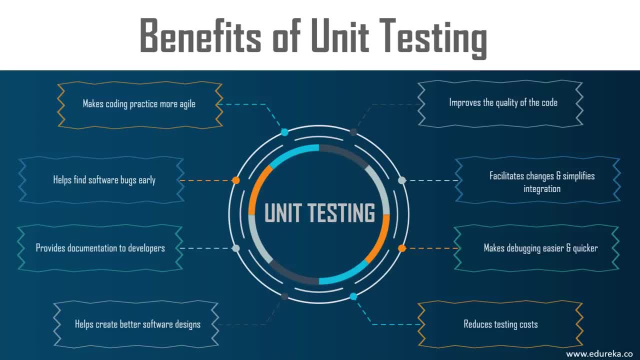 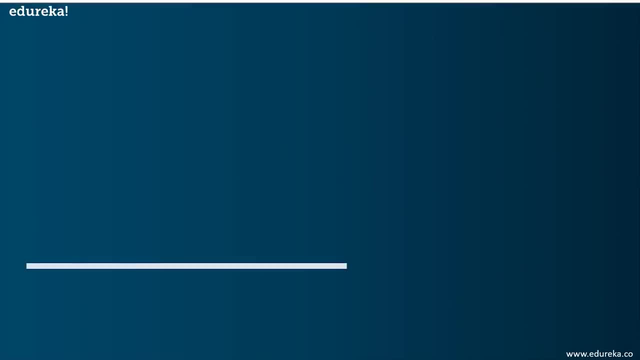 So we have covered the basics of unit testing. If you have any queries regarding what we have discussed and now, please to post them in the comment session and we'll get back to you as soon as possible. So, moving on, let's do a simple demo on how to write unit test. 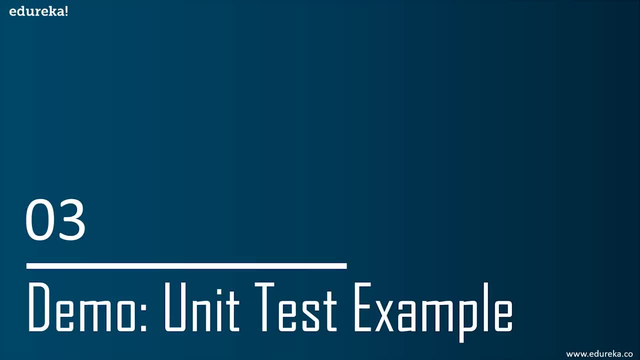 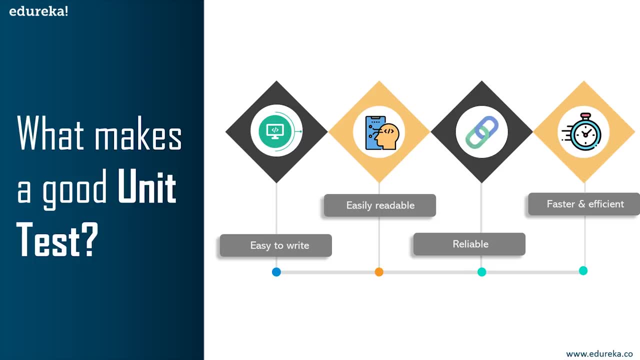 But before diving into the main part of this tutorial and writing unit test, let's quickly discuss the properties of a good unit test. unit testing principles demand a good test is easy to write, It's easily reliable, It's readable and faster and efficient- so easy to write. developers. 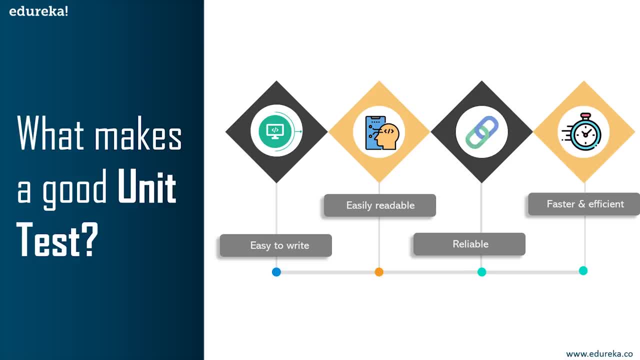 typically write a lot of unit test to cover different cases and aspects of application behavior, So it should be easy to code all those test routines without much effort. It should be readable. the intent of unit test should be clear. a good unit test tells a story. 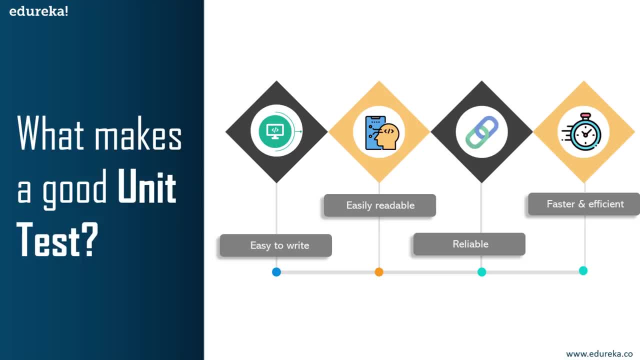 about some behavioral aspect of your application. So it should be easy to understand which scenario is being tested and if the test fails, it should be easy to detect the bug without actually going through the entire program. That's how easily readable your unit test should be. 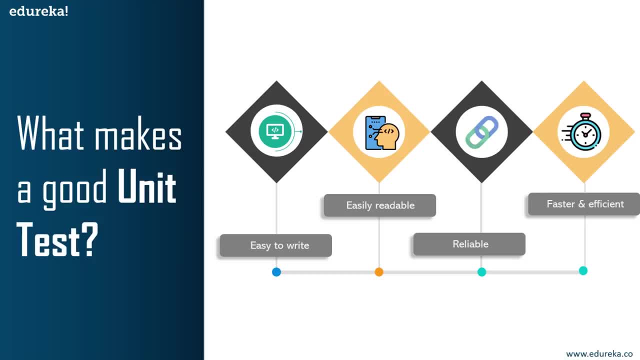 So with a good unit test we can fix a bug without actually debugging the code. then it should be reliable. unit test should fail only if there's a bug in the system under the test. Well, the thing is, programmers often run into an issue when the test fail. 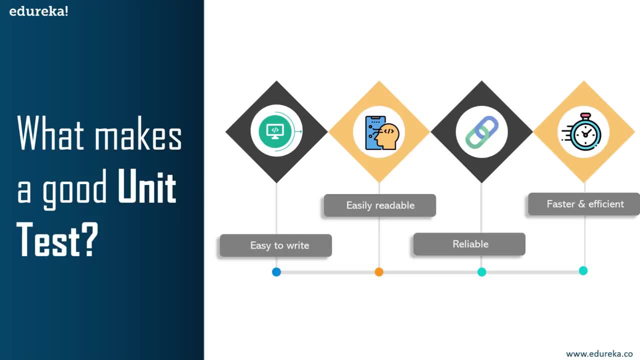 even when no books are introduced. So good unit test should be reproducible and independent from external factors. Lastly, you write your unit test so that you can repeatedly run them and check that no books have been introduced. If your unit test is slow it will affect the final product once load test won't make 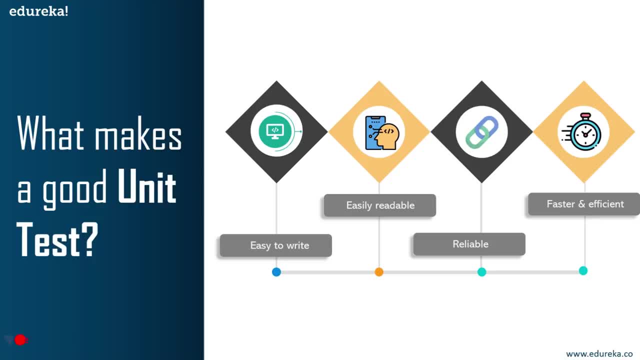 a significant difference, but add 1,000 more and we're surely stuck waiting for a while. slow unit test models indicate that either the system under the test or the test itself interacts with external system, making it environment dependent, which is not a good thing. 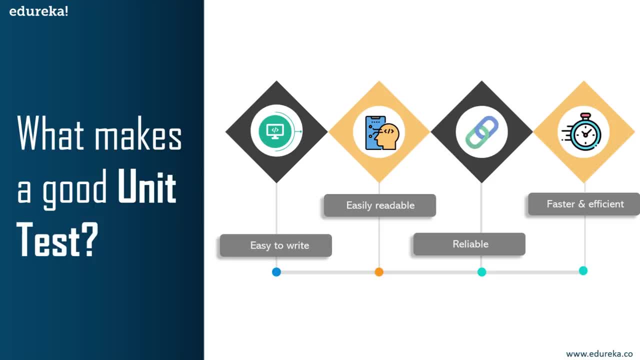 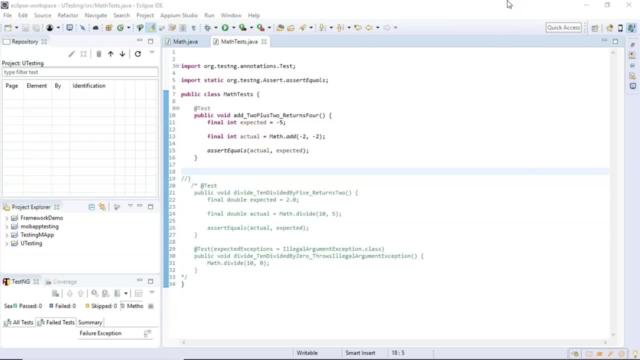 And unit testing. so that's it, guys. There are no secrets to writing unit tests, So let's go ahead and write one. So, guys, before we actually start with the simple demo, There's certain things which you should know. first of all, to perform this demo, you need ID. 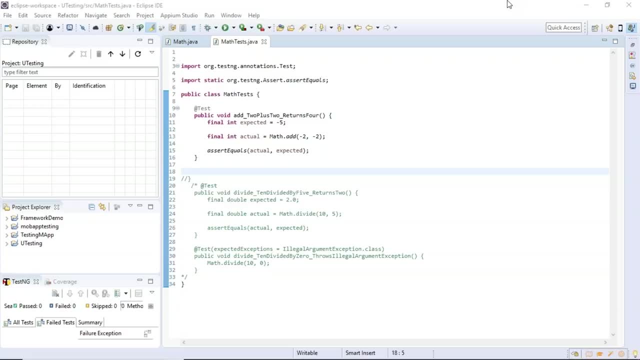 It could be your Eclipse or IntelliJ, anything that you're comfortable with, and you need a unit testing platform, or you can say framework in here. in this demo I'm using a framework, a popular framework for Java, called test NG. There's another one called J unit. 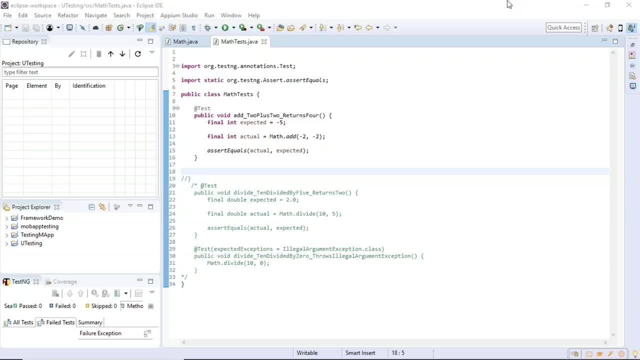 You also have different frameworks for different languages that you can use. will discuss about the unit testing frameworks later, But as for in this demo, as you should know, I'm using Eclipse ID and I'm using test NG for my unit testing framework. So that's all you should know. 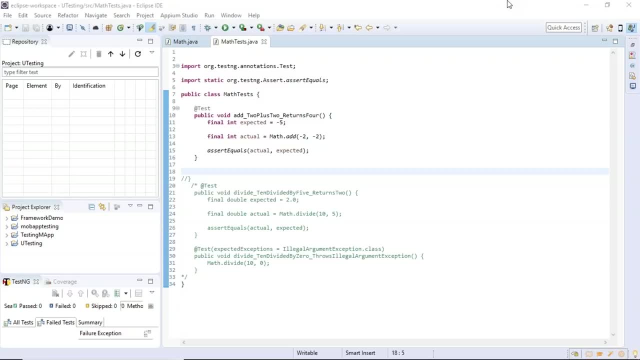 and regarding how you should install test NG. There are different ways. You can install it using Maven. the easiest way in Eclipse is you can actually install it using Eclipse Marketplace. Well, you have help command here. You can see the menu. you can go for Eclipse Marketplace here. 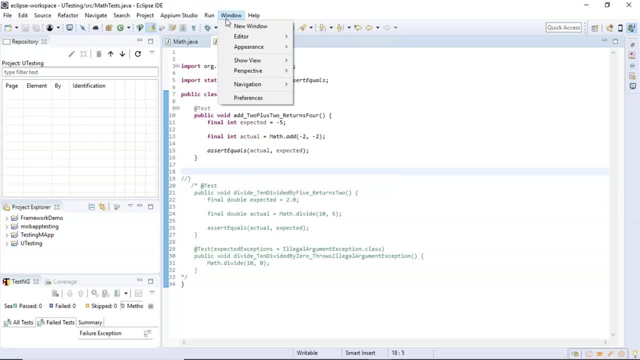 And click for test NG and just click on install. after you've done that, to make sure it's installed properly, All you have to do is go for show you here and click on other and, under Java, make sure that you have test NG installed here. 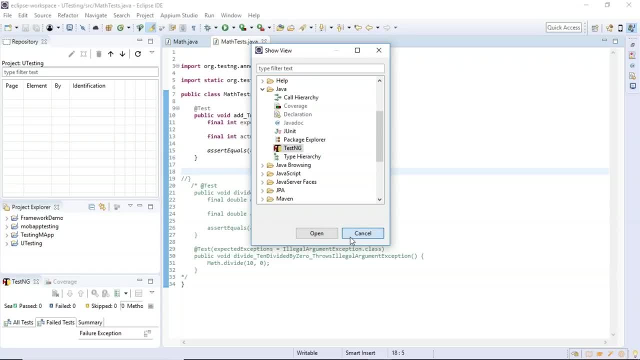 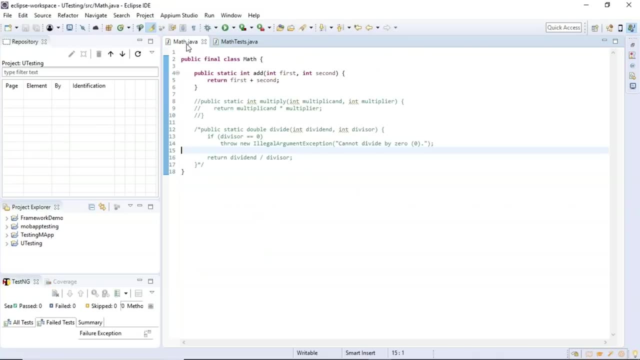 If it's showing test engineer, it means that installation has been done properly. So that's all, guys. I've already written program. Well, it's a very easy program. as you can see, I have a math function first of all, and it has one method which adds two numbers. 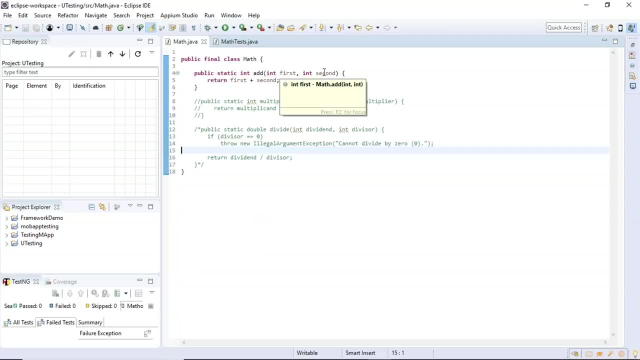 So it's returning into value and I have first parameter in the second parameter and I'm adding and I'm returning the value to my testing function. So this is my basic function and I have a test function which is conducting the test here. So, as you can see, I'm using annotations here. 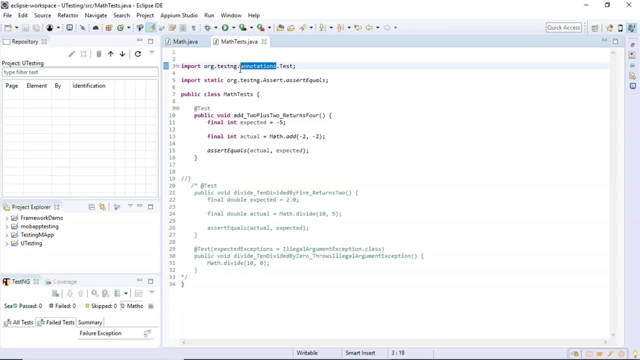 and importing this because to perform test- since I'm using test NG- I need to import these details. So I'm using annotations, which is at test- This is called what we call annotations- and I'm using a method called assert equals, So I'm importing that as well. 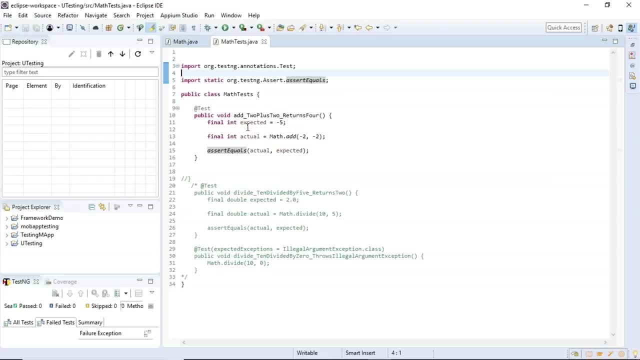 So again, this class contains a single method which is adding two numbers. I have two variables here. One is expected, and actually expected is the one which you want the method to return to, and the actual is the one which actually the method returns to you. 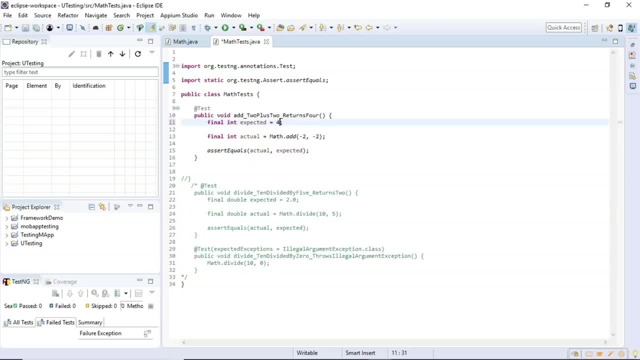 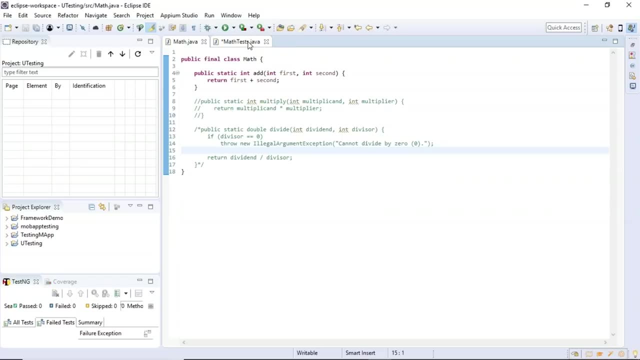 So, as you can see, the expected value I'm giving it as, let's say, four, and as for the actual value, I'm using a math add function which I've created here. as you can see, I have add function here and I'm sending two parameters, which is two and two. 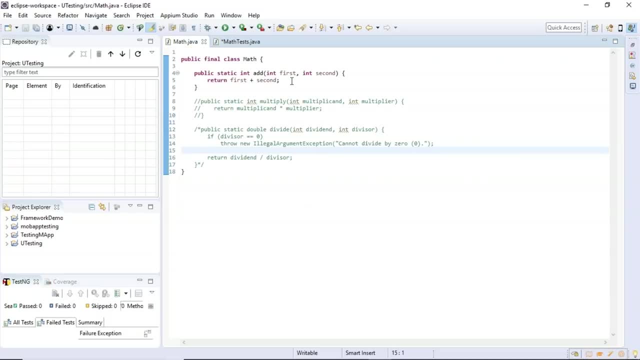 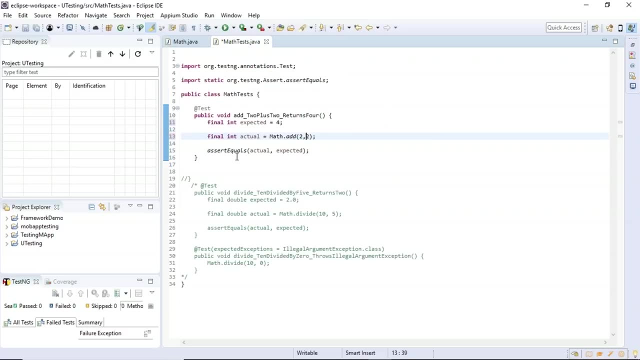 So if I go back to function, since I'm calling this function, the parameters here will be: first is also to, second is also to. so if 2 plus 2, it should written for- and here I have a method- assert equals. this is the actual value which I'm getting from the math function. 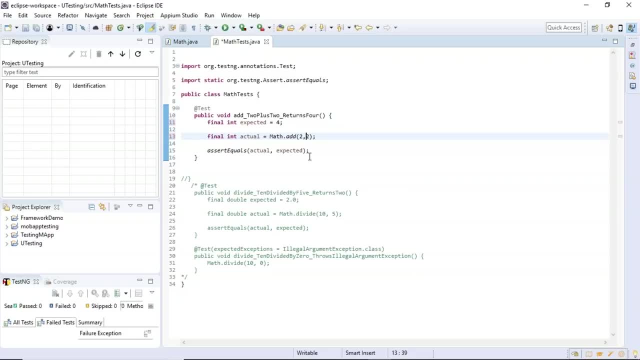 and is the expected value which I've given it for, and since both are for the test, should result success. Let's go ahead and check it. It's as easy as that, guys. So this is one unit of your entire program. You can keep adding units in this way. 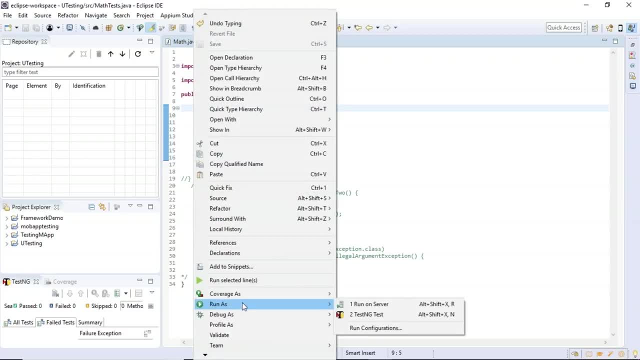 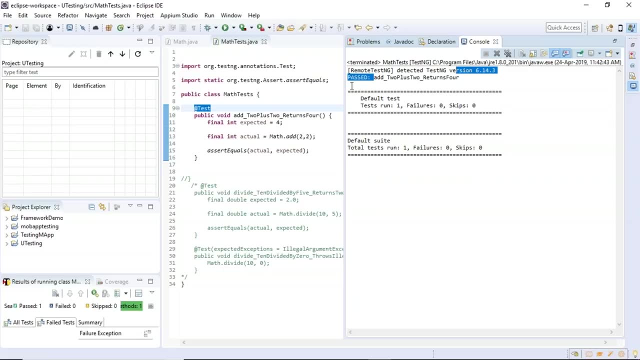 So first we're checking if this unit is working properly. For that, Let me run the test. As you can see, it says this test has passed and the test run. one failure: 0. skip 0. it works right. Let's go ahead and check another: father values. 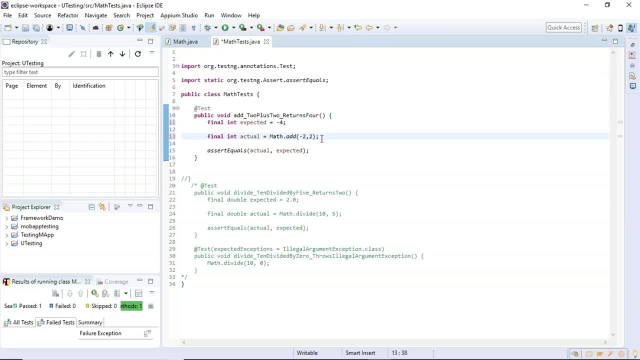 Let's say, let me give it as minus 4 and minus 2 plus 2. that should be. let me just give it as minus 3.. So minus 2 plus minus 3 should be minus 5. now, if I call asset equals function, the expected value is minus 4. 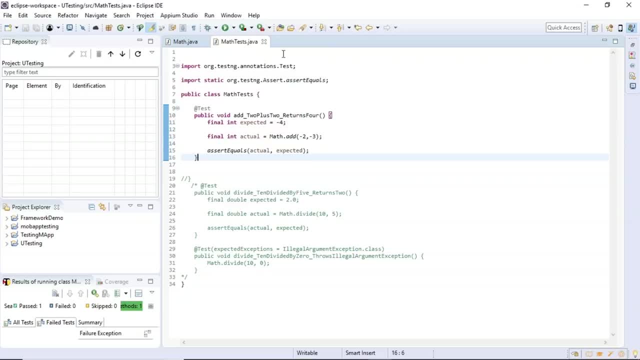 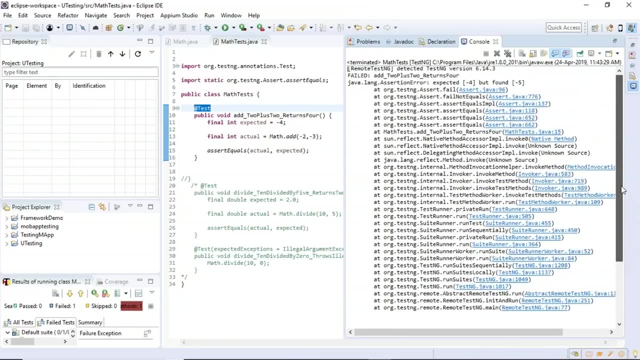 and the actual value is minus 5.. So the test should written failure, Let's go ahead and check it. So here, as you can see, it's giving a long message. It says: this test is failed because expected values minus 4, but the actual value is found to be minus 5. 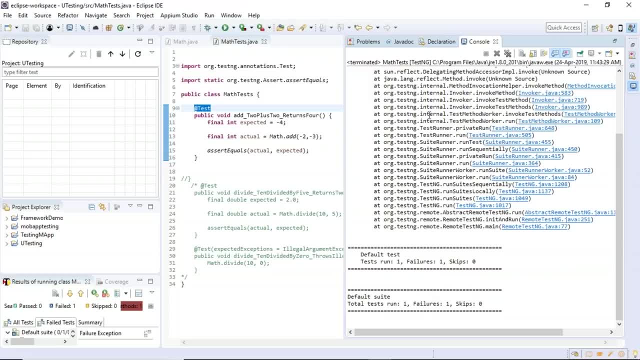 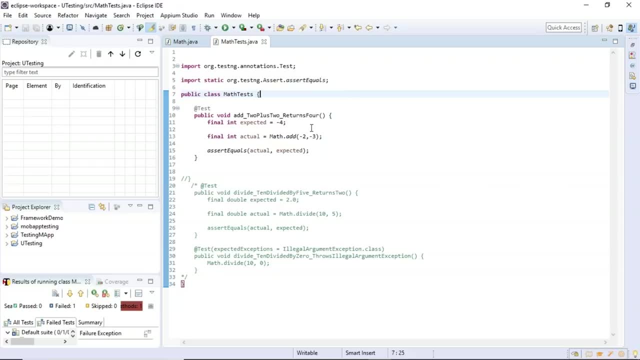 and, as you can see, in the default test, one test was run. You have one failure and zero skips. That's it, guys. And now let's make it a little more bigger, as in: let's add one more function in the math function. I have a multiply function here. 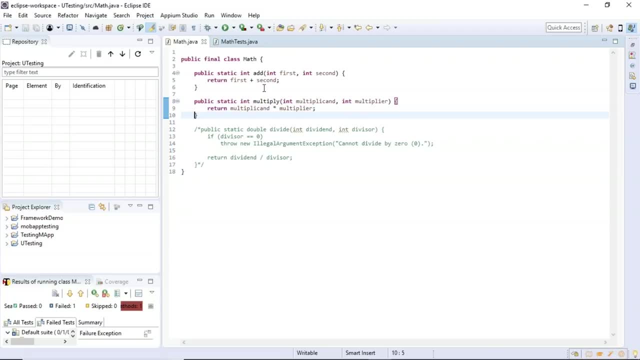 So let me go ahead and add it. So I'm not negating or I'm not commenting that function. Let it be there. It's going to give us result for both the functions here. So this multiplier function, again it's taking two parameters, one is multiplicand. 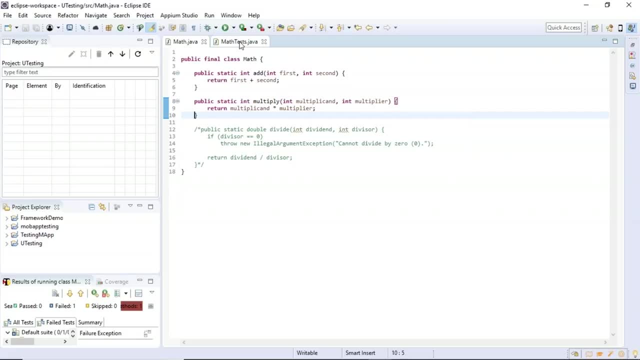 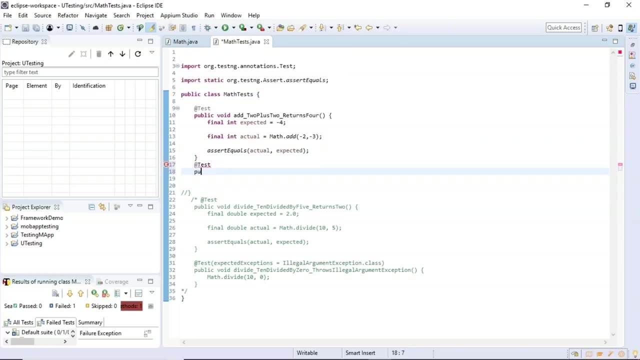 and one is multiplier. It's multiplying them and returning the answer to us. Let's go to math Java test here. I don't have a test annotation for that right, So let's go ahead and write one. So public void: Multiply two numbers. 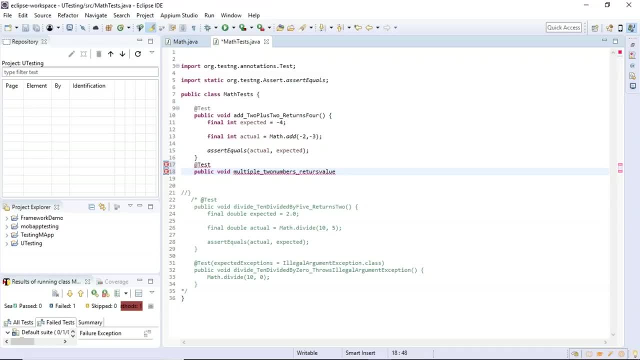 Return some. any name of your function could be according to your wish. and here I go. So final int expected, Let's give it four. Let's keep it simple for a while and then we'll make it complicated, final and actual. So multiply can. let's give it as two. 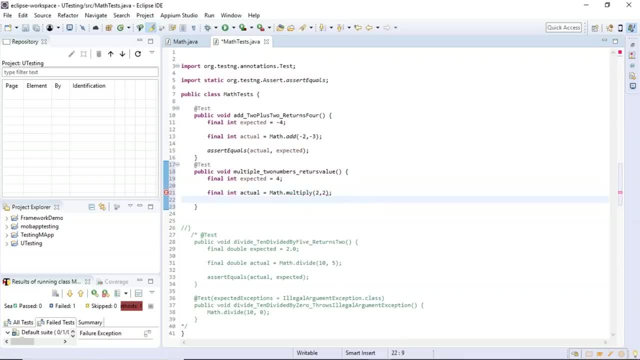 and the multiplier. also, let's give it as two Assert equals Actual and expected. Okay, let me save it. So obviously, the add function: it should result of failure and multiply it should later the correct value. So let's go ahead and test it. 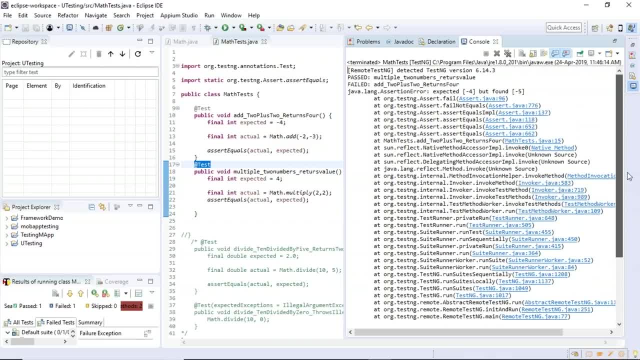 So, as you can see, to test a performed one failure. So let's go ahead and see. it is multiply two numbers has successfully passed, but add has failed because expected values minus four but it was found to be minus five. So that's how you write unit test. 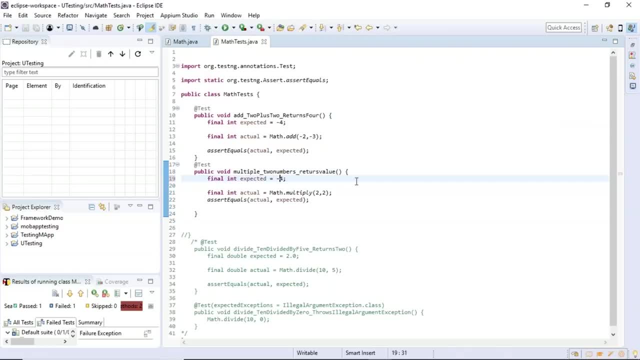 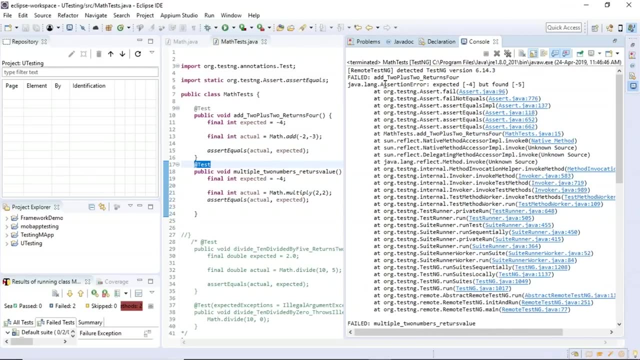 Let's make it minus four and check if it's working for the negative numbers as well. As you can see it showing two failures here. both are multiply function and add functions have failed. So, guys, it's as easy as that. first I wrote a unit test for add function. 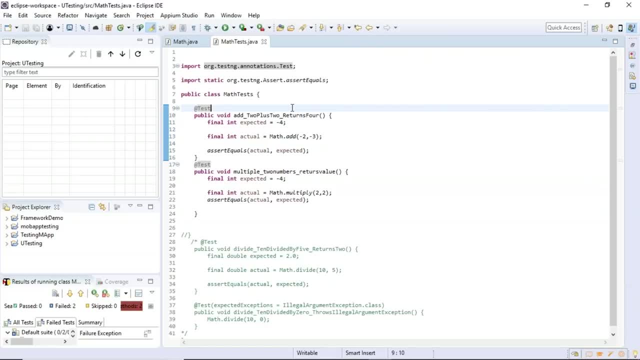 So that's add function is a unit. You can call it a unit, a part of your program, and I've checked and tested. since the method is working properly. I'm going one step ahead and added one more unit, which is a multiply function. Even it's working properly. 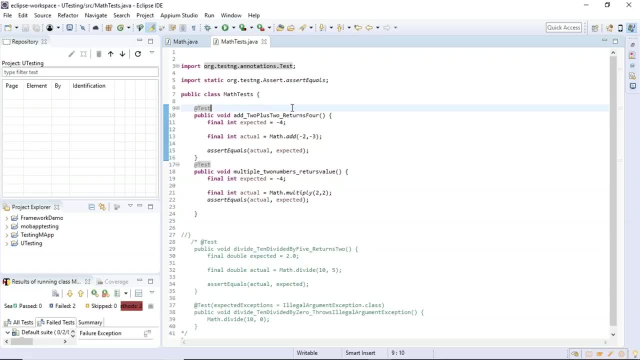 Then you go ahead and add one more part of our more unit to your function or the program of your application. So, guys, that's how you write simple unit test. as you can see, the tests were very simple and these are very basic level test. 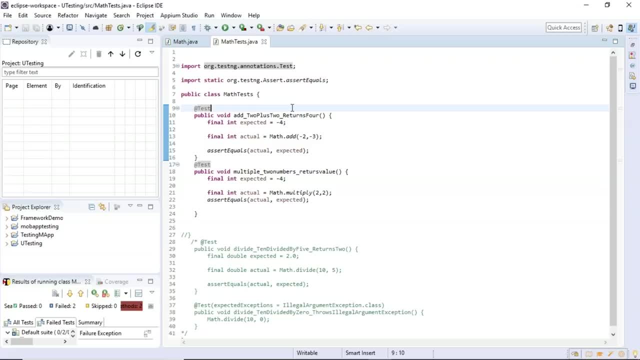 You can go ahead and make, explore and make them complicated, So I'm not going to do the divide function. the purpose of this demo was for you to understand how simple it can be and how your unit test should be not very complicated. There should be very easy to understand one. 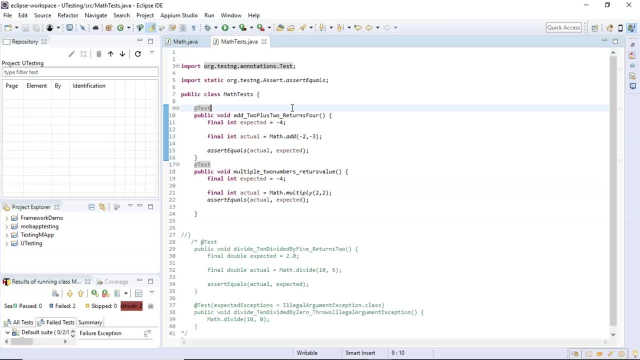 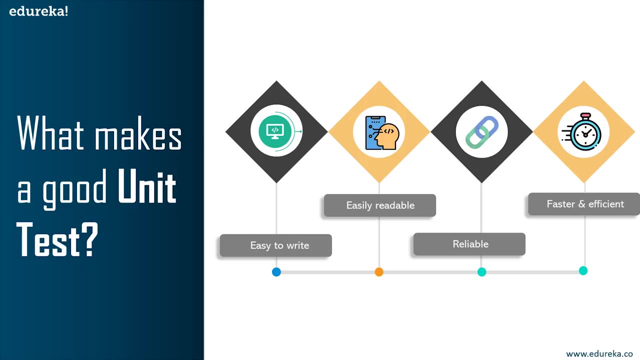 Look at it, the person who is looking at your coach understand what your code is actually performing. So there you go, guys. That's how you write your unit test. Let's get back to the theory part. So I hope you have understood what we did in the demo. 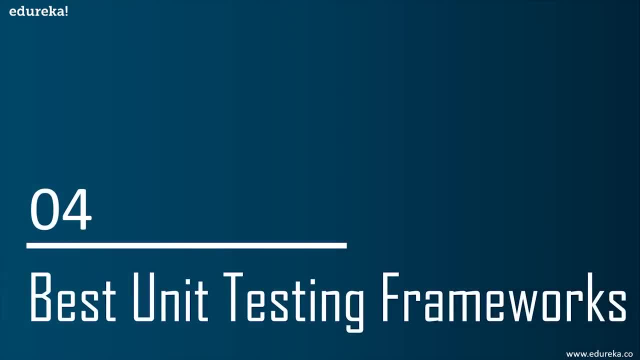 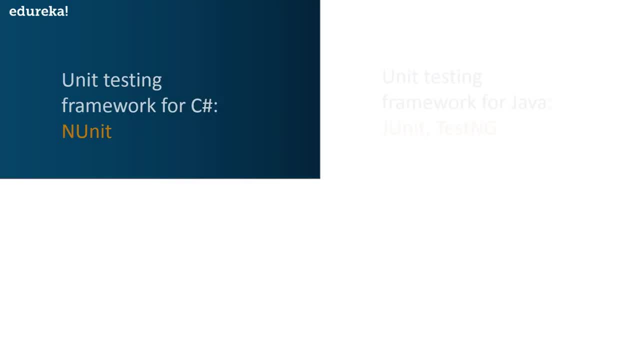 Let's move forward and check out the most popular or the best unit testing frameworks to automate unit tests. So the unit testing framework for C sharp is n unit and unit is a unit testing framework that belongs to X unit family and it's written entirely in C sharp. 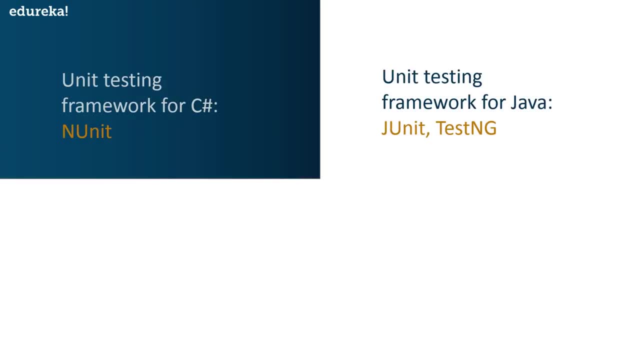 Now, as for Java, you have many. the most popular ones are J unit and test in G. J unit is basically an open-source unit testing framework for a test-driven development environment. We call it TDD. It's opposed the core concept of first testing, then coding. 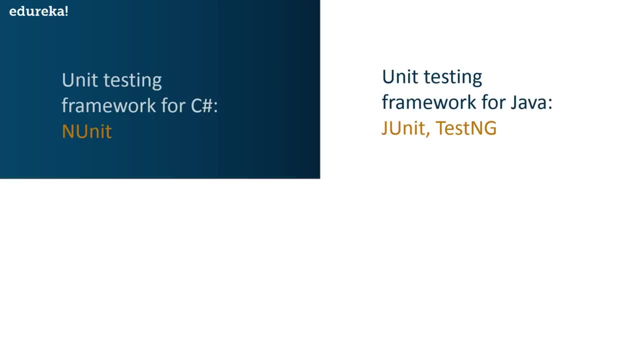 this framework is specifically designed for Java programming language. in this, data is first tested and then it is inserted in the piece of code, So it provides the simplest approach for writing code very swiftly and easily. it also offers annotation for test method identification, as we did in the demo part. 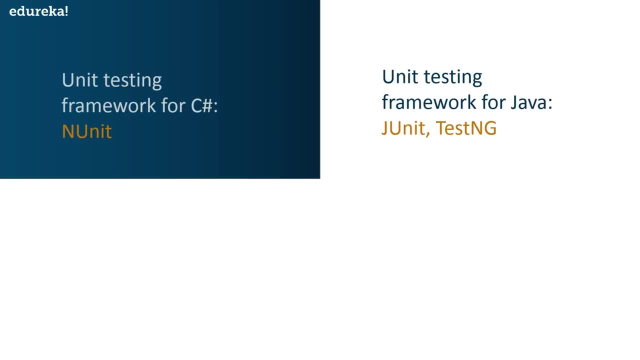 We use test in G and I've showed you how to use annotations and an asset equal function. moving on, A unit testing framework for C and C++ is M unit. It's an open-source unit testing framework which is designed for software application. 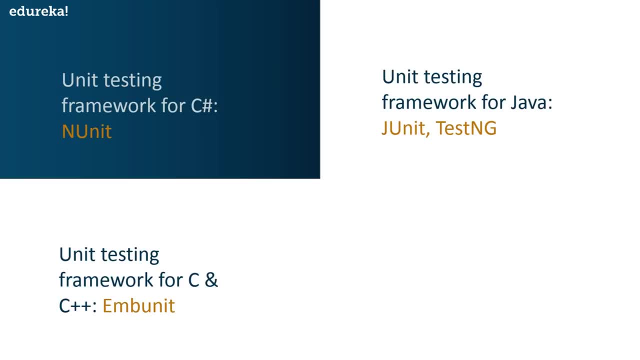 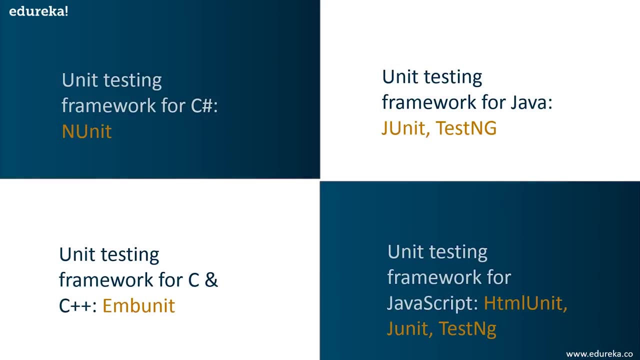 which is written in C or C++. Well, it's used by both developers and testers for software applications, which are written again in C and C++. So next we have unit testing frameworks for JavaScript. as you guys know, JavaScript is the language of web. 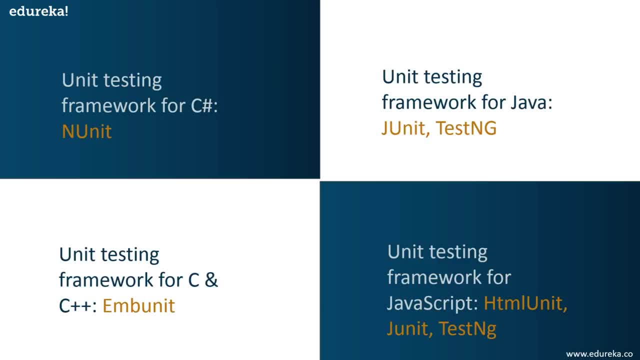 which is the reason there are large number of test automation frameworks that support Java JavaScript, So here's one of the most popular unit testing framework for JavaScript. It's called HTML units. It is an open-source unit testing framework that supports JavaScript and it provides graphical user interface features like forms. 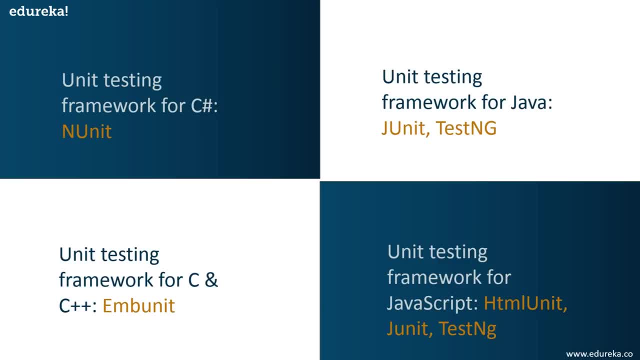 links, tables, etc. It offers an open-source Java library which contains graphical user interface- less browser for Java programs. It also supports cookie submit methods like get post and proxy server. It is used for testing applications that are used within frameworks like J unit and test entry. 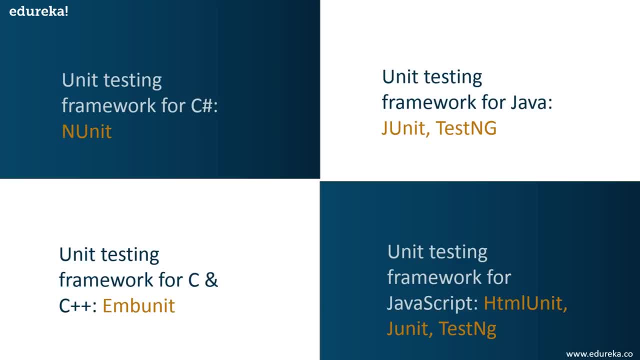 So right, these are not the only ones which are there in the market. There are many other popular frameworks, but these are the top unit testing frameworks which support different languages. as we discussed for C sharp, It's an unit for Java, You have J unit and test in G for C and C++. 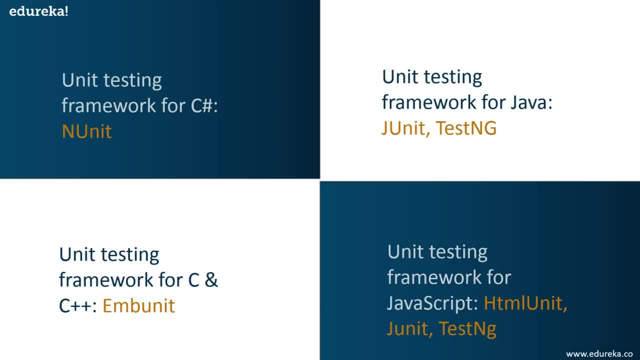 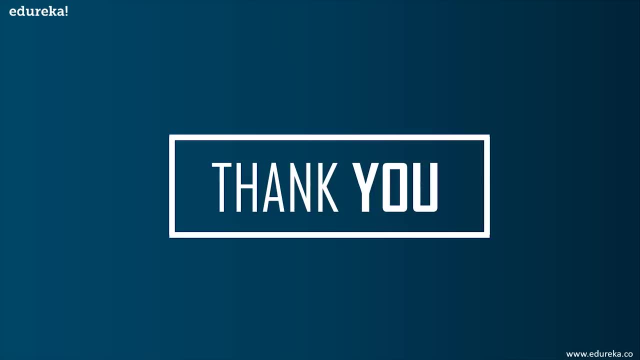 You have MB unit for JavaScript, You have HTML unit, J unit test engine, many others. So if you want to know more about them, you can go ahead and research on them. So, guys, with this we have reached the end of the session and I hope the session was interesting. 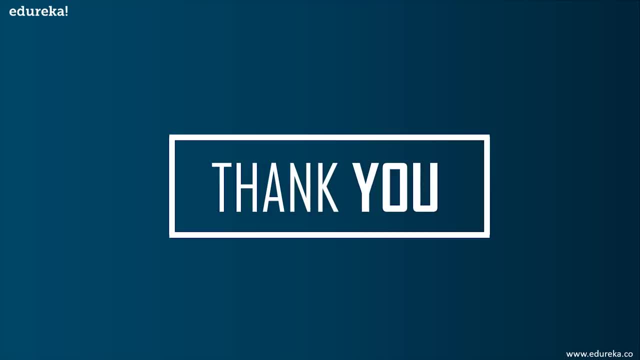 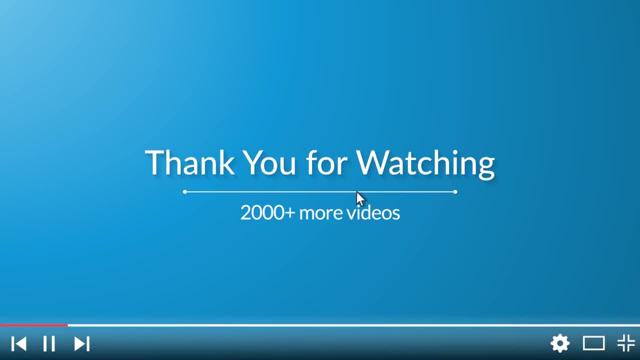 Well, if you have any doubts regarding the demo or any theory part, please do post them in the comment session and we will get back to you as soon as possible. Thank you, guys. I hope you have enjoyed listening to this video. Please be kind enough to like it.